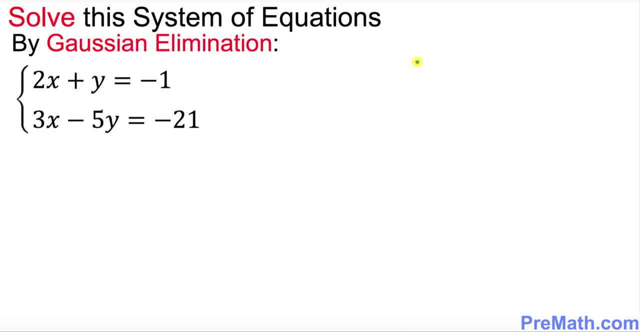 Hello again everyone. In this video tutorial we are going to solve this given system of two equations with two variables by Gaussian elimination method. This method is also called Gauss-Jordan elimination method. So let's go ahead and get started with this method. I want 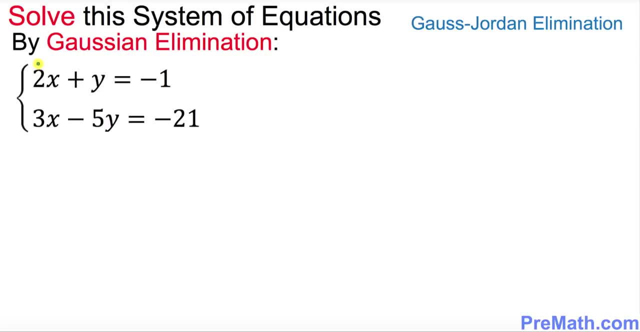 you to look at this system of equations. Look at the coefficients. Over here the coefficient is 2.. Here no coefficient means by default it's going to be 1.. Here is a 3 and here is a negative 5, and on the right hand side numbers are negative 1 and negative 2.. Now I want to transform. I want 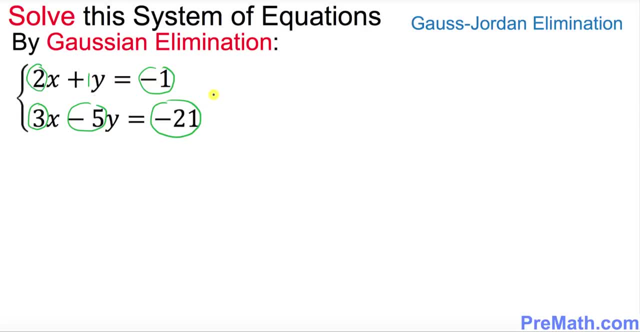 to put this system in a matrix form. So let's go ahead and put in a matrix form. It's going to look like this thing. We have to be a little bit careful, Okay, so I'm going to put a right here. the dot dot starts over here. Put down the numbers, which is: 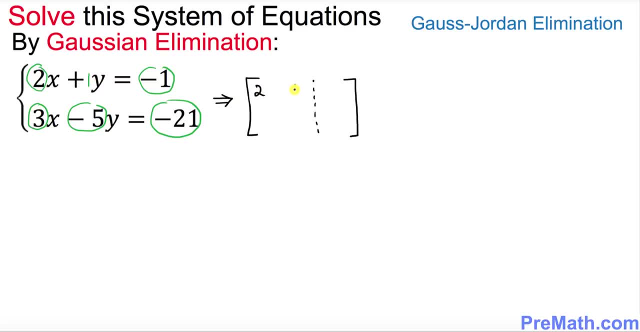 2: 1, 3, negative, 5.. 2: 1, 3 negative, 5 and negative, 1 and negative 21 is going to be right up here. By the way, this matrix is called is called augmented matrix, And our now objective is our objective or our goal is to make sure that our this augmented matrix. 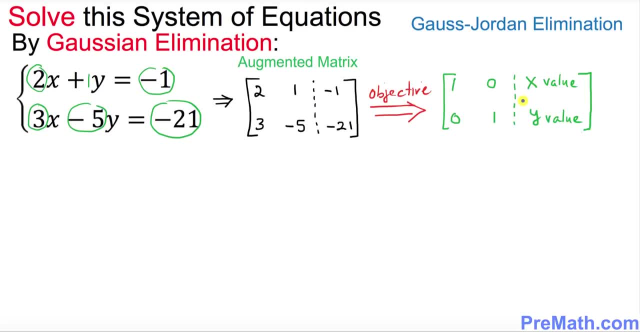 must look like this kind of matrix where we have ones only on the main diagonal. the rest are zeros. If you can see, this means that ones are only on the main diagonal. You can see that thing. and on the right hand side we're going to have X value and Y value. 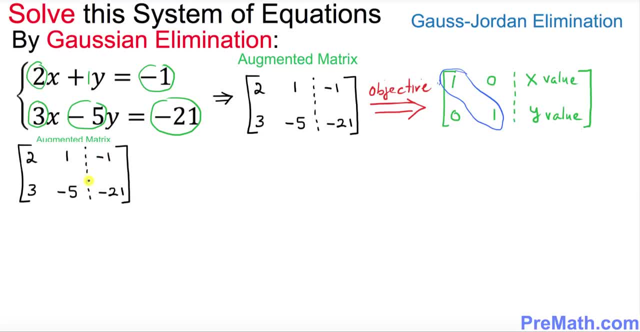 So here I have put down my augmented matrix right up here. Now our goal is, as I mentioned before. we want to make sure that we should have this form. This number should be supposed to be a 1 0, 0, 1.. To achieve that goal, we're going to perform some operations. So these operations I'm going to do. 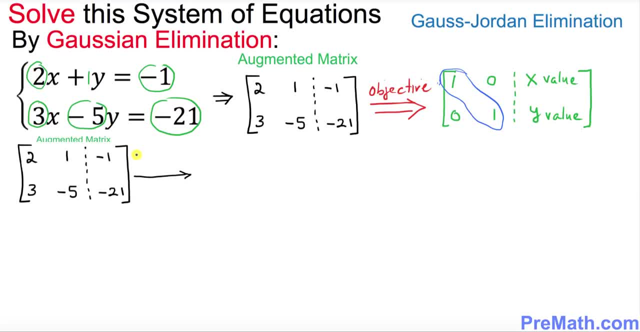 The very first operation is going to be: I'm going to multiply the first row, the top row, row number one, multiply by 3 with row 1 and put it back on row 1.. And at the same time, I'm going to multiply the second row by. 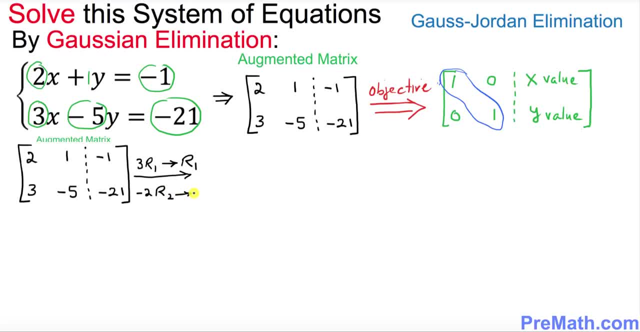 negative 2 and put it back to second row. So our this matrix is going to look like this This matrix is going to look like: So the matrix is going to look like 6, 3, negative 3 and over here it's going to look like negative 6, 10 and 42.. 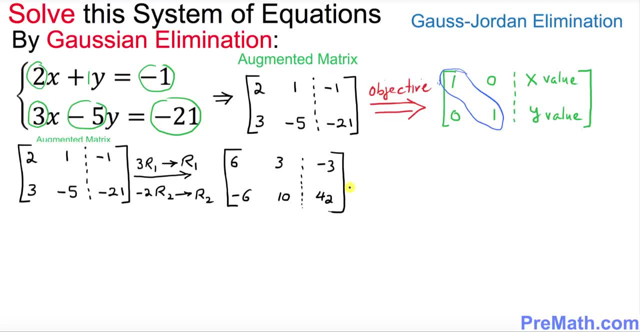 So far, so good. And now the next thing, what we're going to do, is the next operation we're going to do, Is: I want to add first and second row and put it in the second row again. I'm going to put this. so this is what I'm going to do. I'm going to put down. 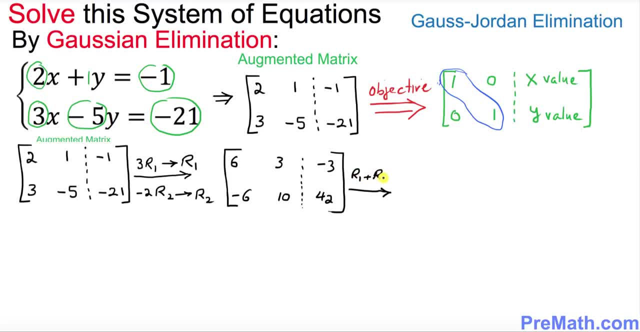 row one and I'm going to add two rows and put it down to a second row, r2.. So our matrix is going to look like this one over here. So this is going to become, on the top six, three and again you have to make sure- and this is going to be a negative 3 and here is going to be a 0, 13 and 39.. 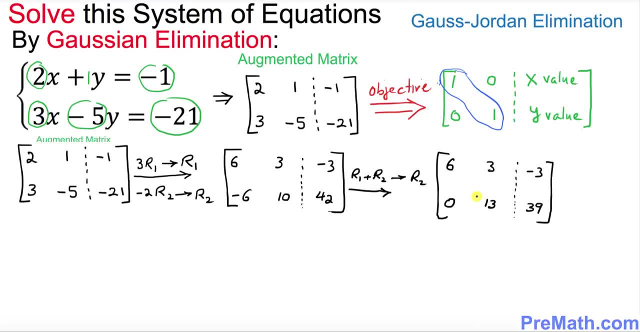 So far, so good. And now, as you can see, the second row. we can easily multiply by 1 over 30.. that means we can divide it. so this is what I'm going to do. next one. so I'm going to multiply row 1 over 13 times. second row, and then row 2 is going to. 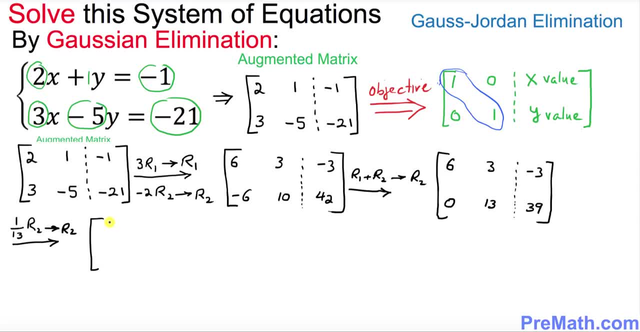 become simply so once again: 6, 3 is going to be same and negative 3 on the top. we not gonna touch that one, and the second row is going to simply become 0, 1 and this becomes 3. so far, so good. so the next one we're going to do is we're. 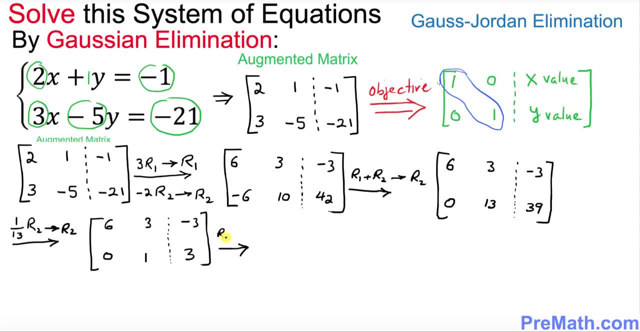 going to say r1, row 1, minus 3 times the second row and put it in a 3 row one, the first row. so that's going to look like it's going to look like six. I'm going to once again, I'm going to put down six, zero negative 12, and this is 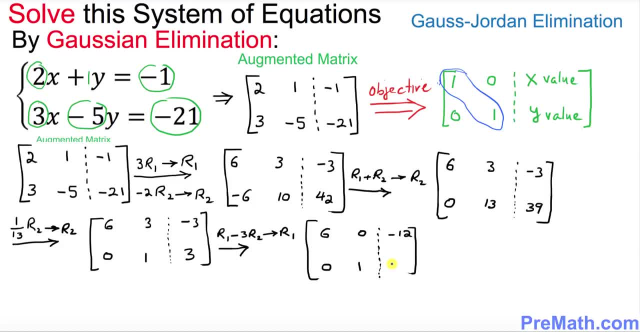 going to stay same: zero, one and three. and now the final step. we are almost finished. I want you to multiply one over six times row one and put it back to row one, so that's going to look like one zero, negative two, and once again make sure. so zero, one and three. so now, as you can see, this is our x value. 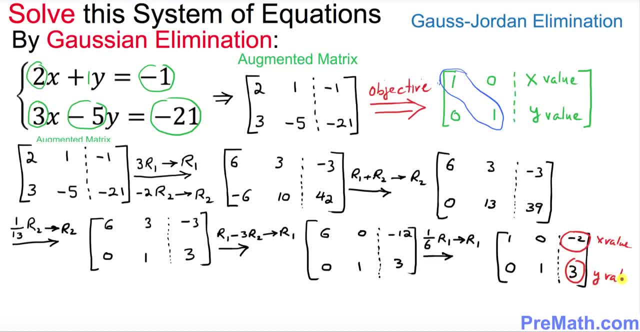 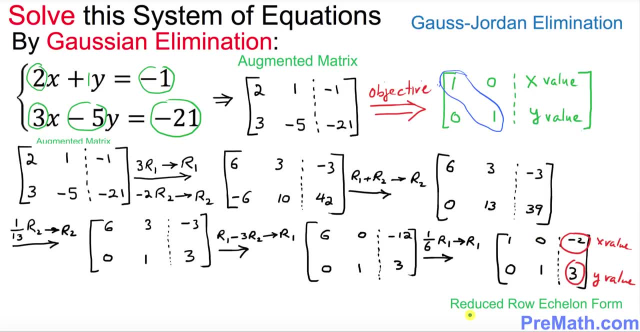 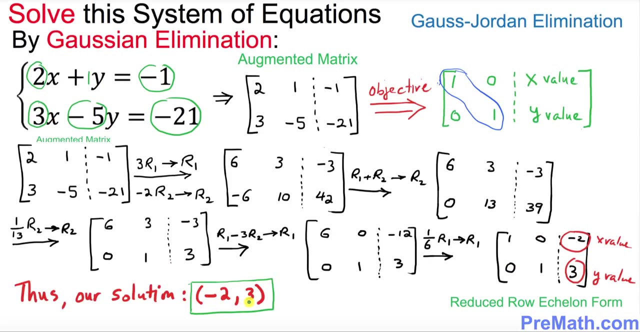 and this is our y value. and one more thing: this one, zero, zero, one matrix. this part only is called reduced row and echelon form. in this means that means is that our main diagonal has ones, the rest are zero. thus our solution turns out to be a negative 2 comma 3, where negative 2 is our this x value. and 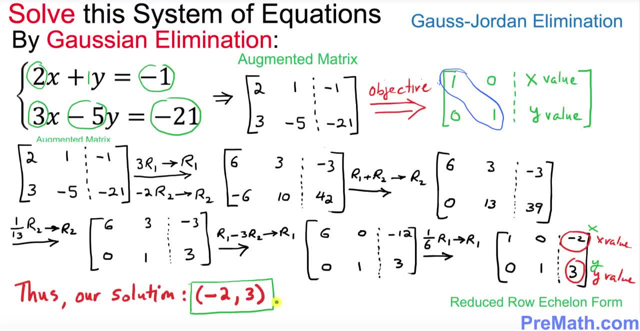 3 is our. this y value. thanks for watching and please subscribe to my channel for more exciting videos.